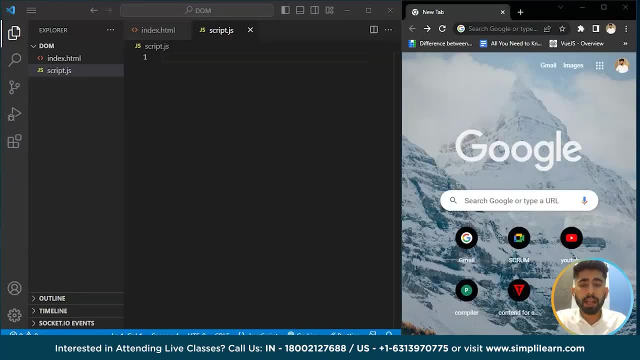 Now let's jump to our video. Let's start this with a quick overview of what the DOM is. So the DOM is a tree-like structure that represents the elements on an HTML page. Each element on the page is represented as a node in a DOM tree. I'll explain it to you in a while. I'll give you an example also. By manipulating the node in the DOM tree, we can dynamically change the content and layout of an HTML page. 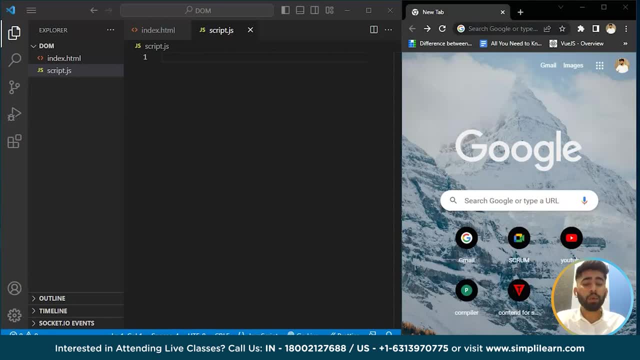 To get started with DOM manipulation, we first need to access the DOM tree. We can do this by using JavaScript document object, And the document object represents the entire HTML document And we can use it to access and manipulate any element on the page. 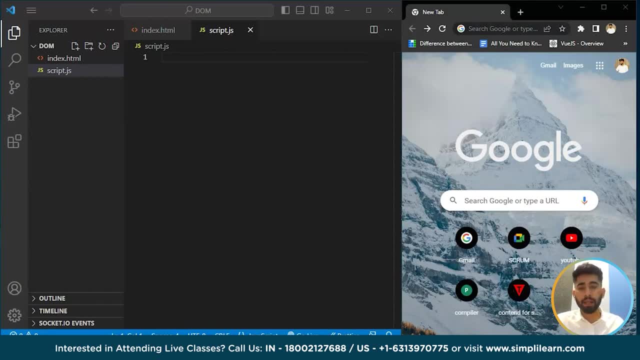 Now, as you know, DOM is like a tree, For example, it's like one document which is an HTML. Then that HTML page is divided into two parts: head and body. Now, inside the head element there is meta tag, then there is title, then comes links and all Okay. in the head part, 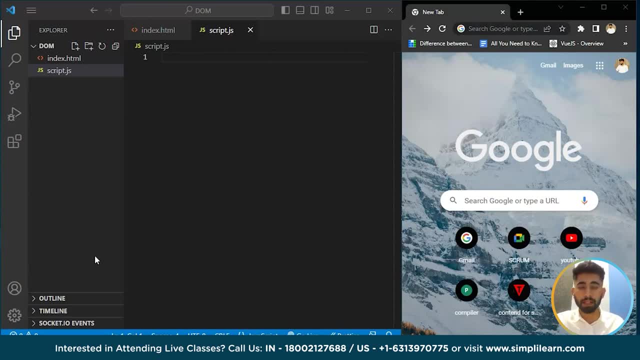 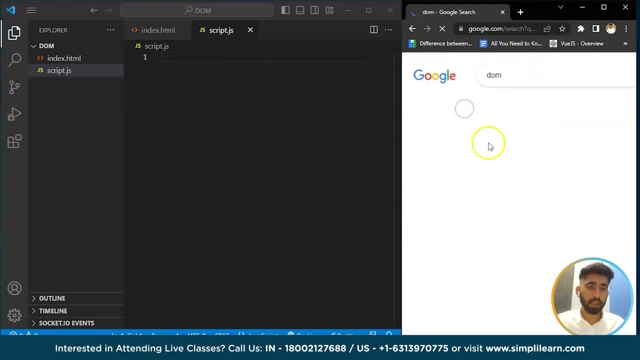 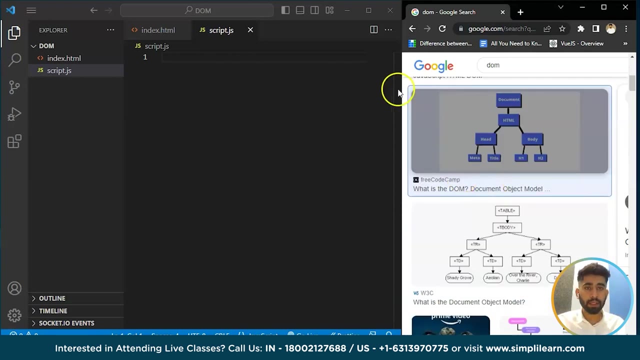 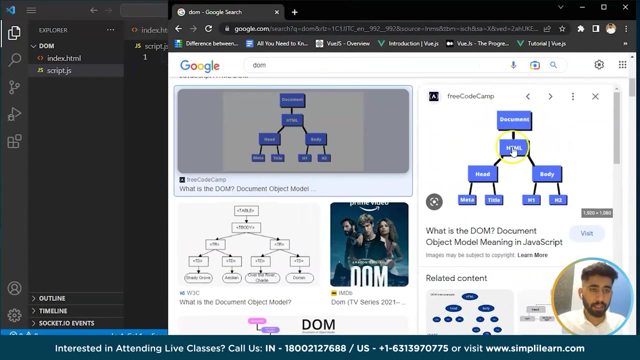 Then in the next node, if you imagine one tree, I'll explain you Just a second. I'll write DOM and inside here I'll find an image. Yeah, So I want to make this image big, Okay. So, as you can see, here there's one document which is a page In HTML. there is head body And in head there is meta tag type. 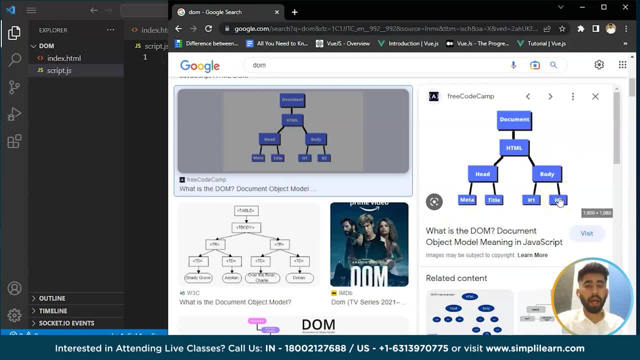 So I'll write DOM and inside here I'll find an image. Yeah, So as you can see, here there's one document which is a page And in the next node there is title links. We add in that head part And in body we add H1, H2, which is heading tags, And we also add paragraph tags and so many other tags. Okay, 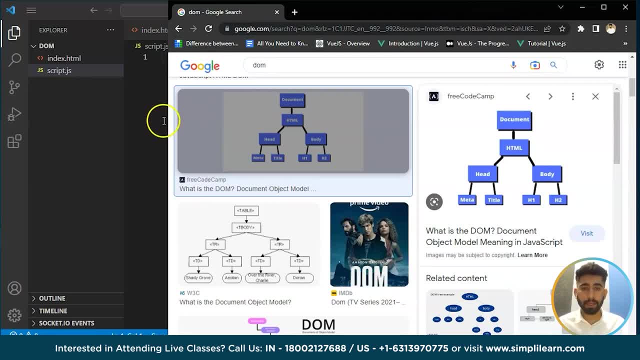 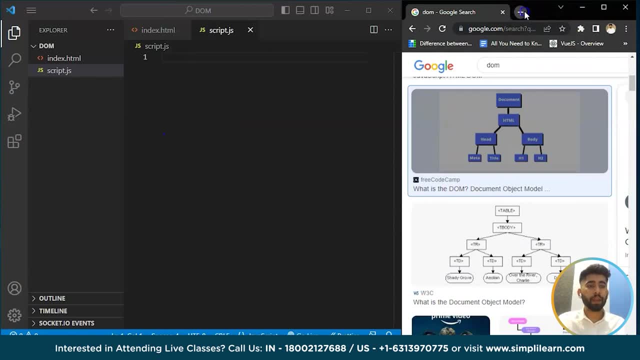 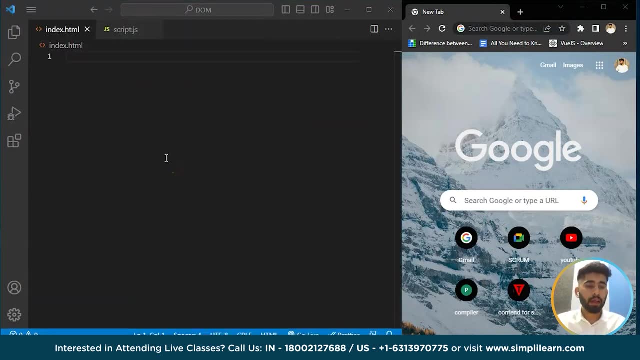 Now we'll work on the document object model And we'll start with adding element to the page. Okay, So let's cut this and start working on. Let's create a boiler code for that. I'll press ctrl and 1, shift and 1. sorry, and there one boiler code is created for us. Here I'll write: DOM manipulation. 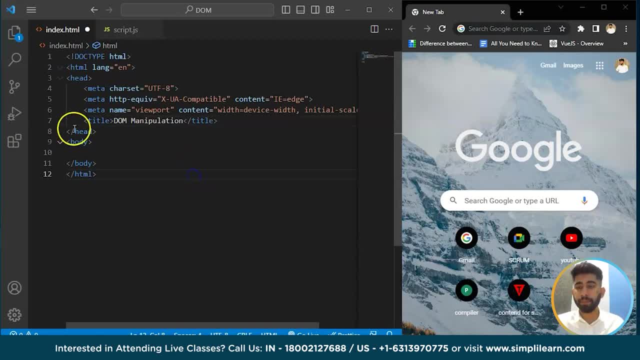 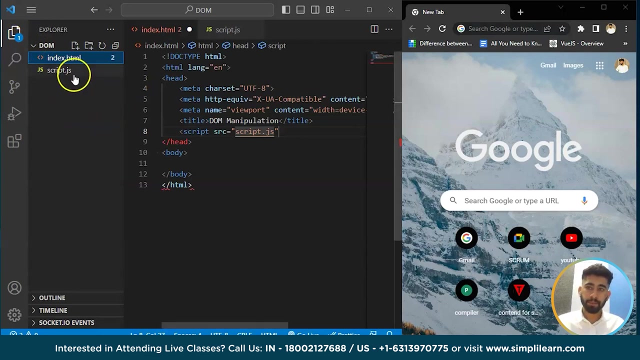 Okay, and here I'll add one script tag. Inside that script tag I'll give a source and I'll give the source as scriptjs that we just created for us. Okay, this file, and here I'll write defer, Because it can defer also. Let's close this one and inside the body I'll write some text for now, to check whether it's working or not. Hello from SimpliLar. 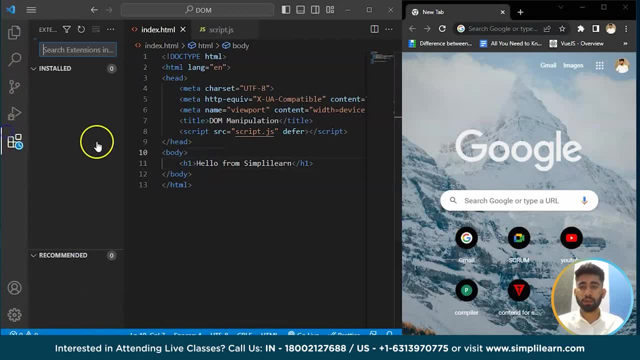 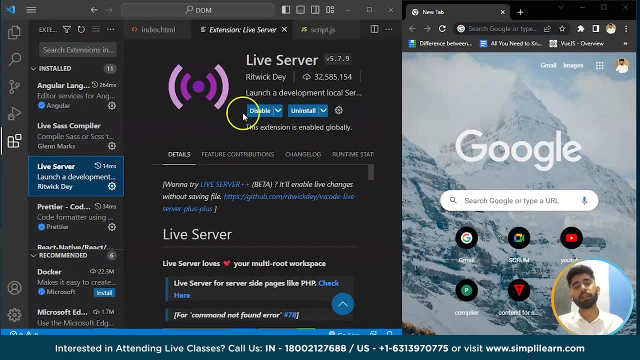 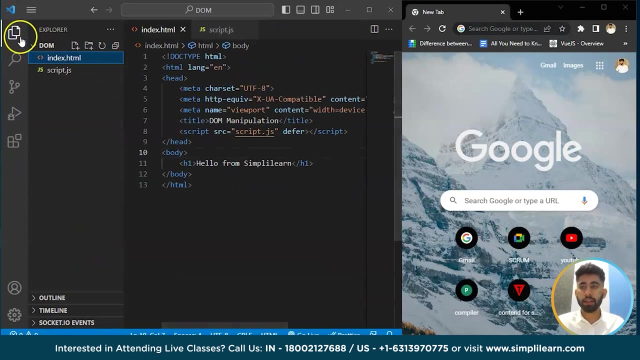 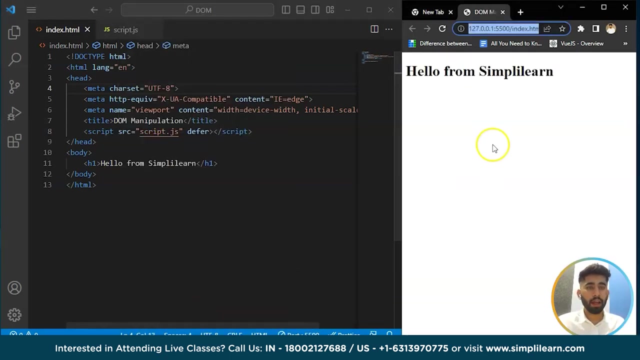 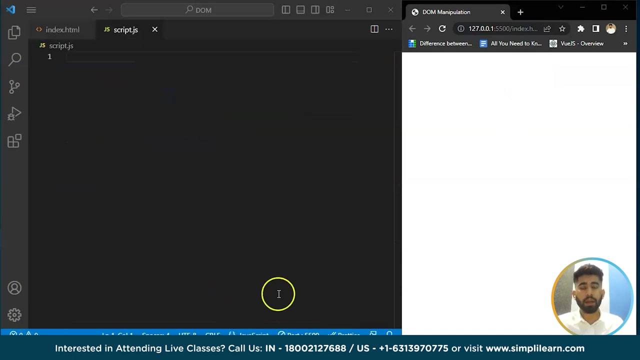 Let's save it, and I've installed this awesome live server extension. You can also install it on your system. It's very easy. Just press here, Install and you'll get installing your system. So after that you can just right click here and here you'll find one option open with live server. Just click on that and one page will get open with the title that we have added, And here is hello from SimpliLar. So page is working completely fine. So there are two different functions to add the elements. 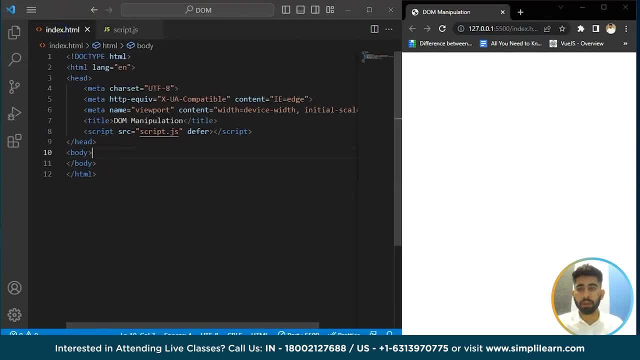 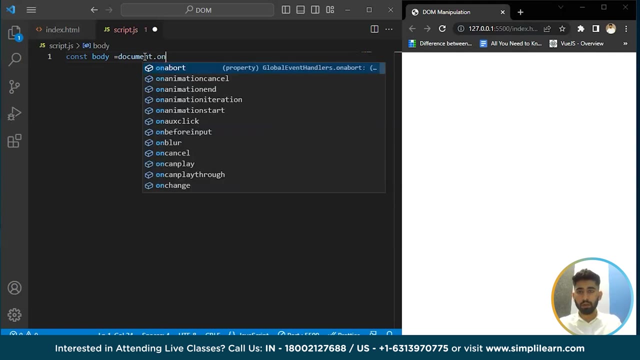 To our page. So let's open the script page And here we'll write const body, And here we'll write document. After that we'll append it. So I'll tell you about this too. So there is one append And, as you can see, 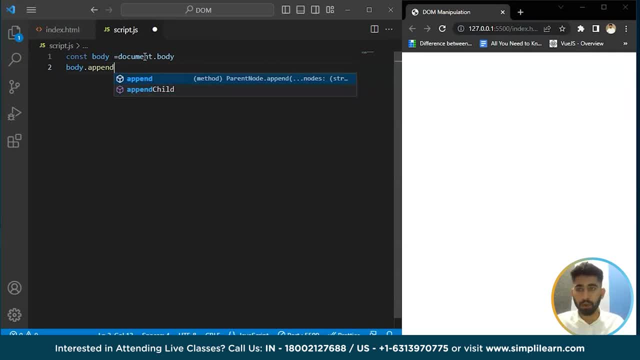 There are two methods: Append and append child. I'll tell you about both of them. So first we'll see about append. first, Here I'll write hello from SimpliLar. So this append only takes up the string elements. Okay, So an append child doesn't take the string, It takes the node. I'll explain it to you in a while. Let's save it And, as you can see, it's showing hello from SimpliLar. 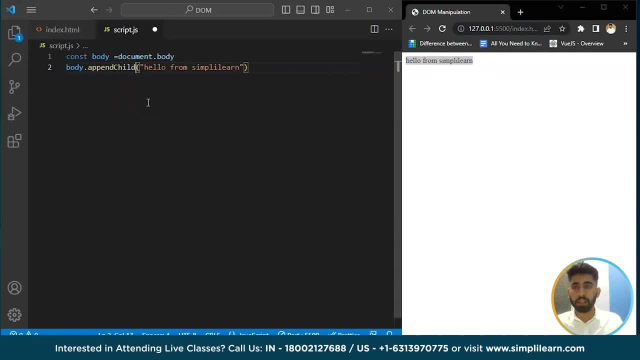 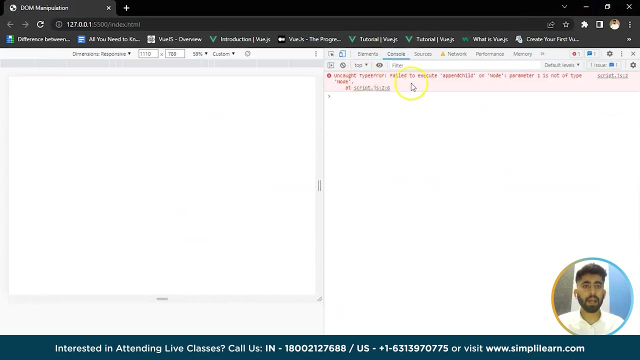 But now I'll write here append child function And whenever I'll click a save There is nothing here. It's because I'll inspect and tell you more about it. Let me open my console first. As you can see, it's showing an error That it failed to execute append child on node Parameter 1 is not the type node So, as I have already told you, It doesn't take the append child. 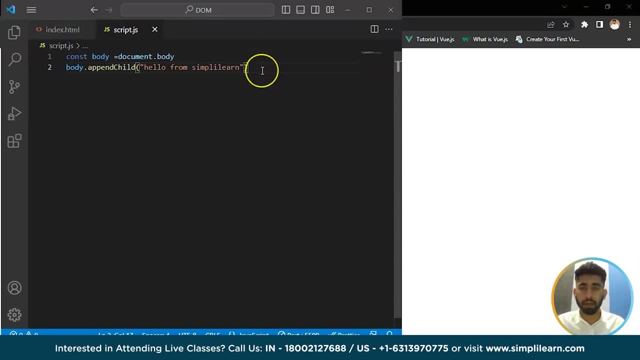 These- both append and append child- works very similar, But I always use append more. Whenever there is a need of append child, I'll use that whenever it's a node and all, But you can also work on append. So this is about how to add the element. Okay, Now we'll see how to create an element. Okay, As we. 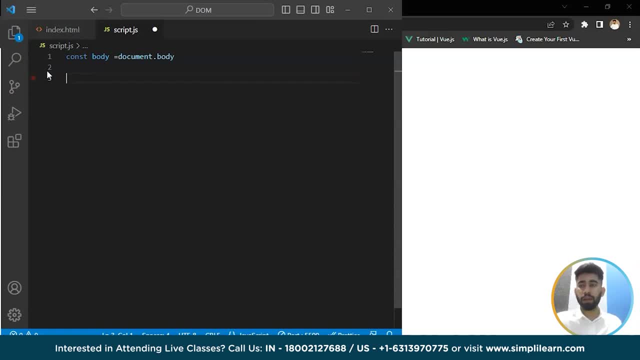 got to know how to add that. now we will see how to create a element for that. we will write document dot. create element will pass the type of element that you want to add. so there are all the type of html tags that we can add. okay, so let's add div here and we will write here. 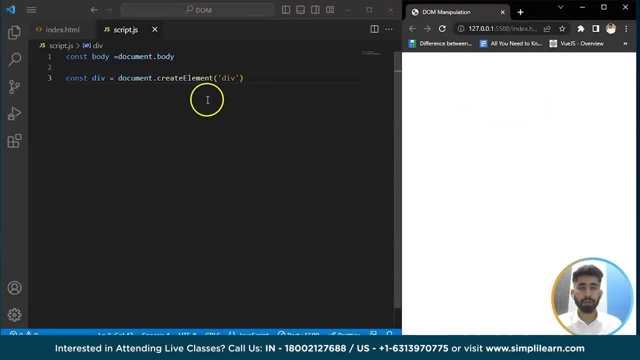 we'll save it. nothing is going to happen, right? we can't find any element, because we have created our element, but we haven't added it inside our main page, okay, so? so creating anything in javascript is very different in creating a page, right? so let's move forward and append the dip. 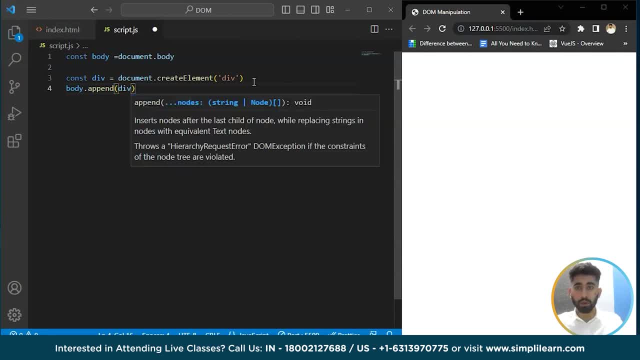 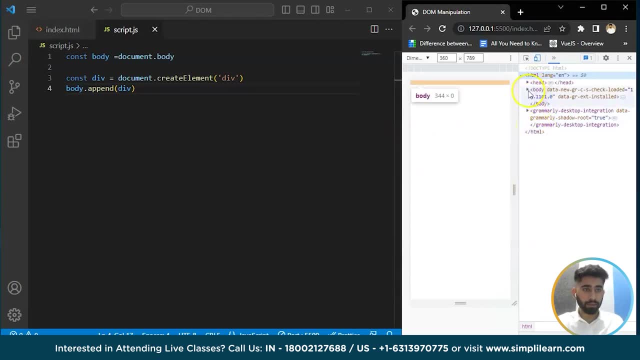 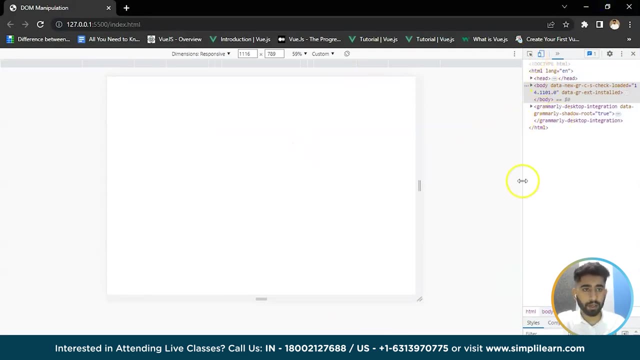 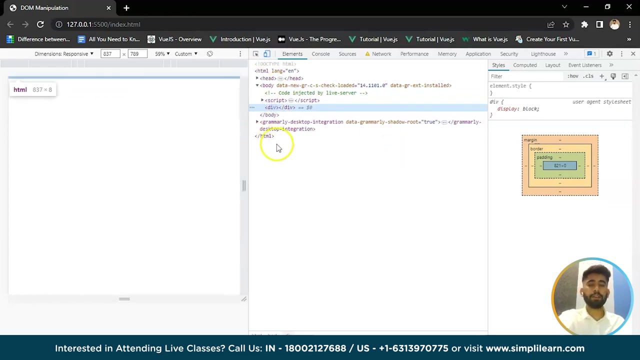 okay, now you will see the dev in the body part, okay, and, as you can see, there you'll find the. let's maximize this page so we can get the now. inside the body, you will find the dev, but it's empty right now because we haven't added anything inside. 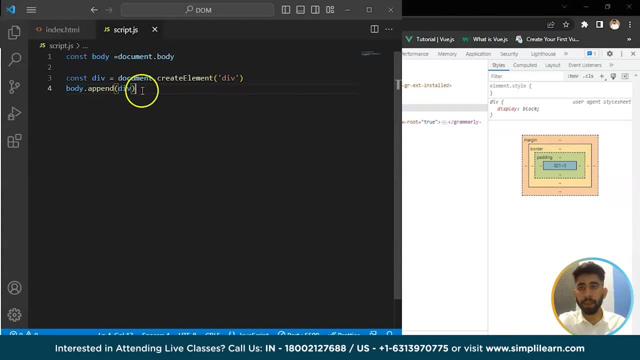 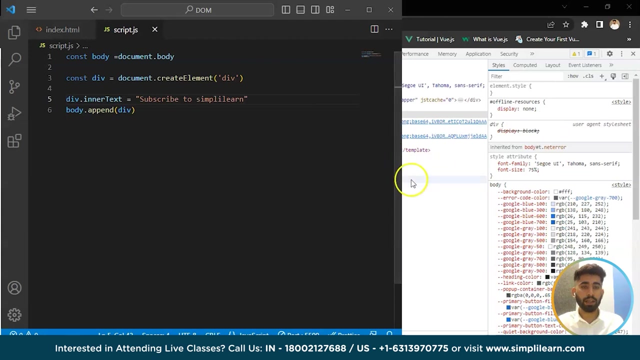 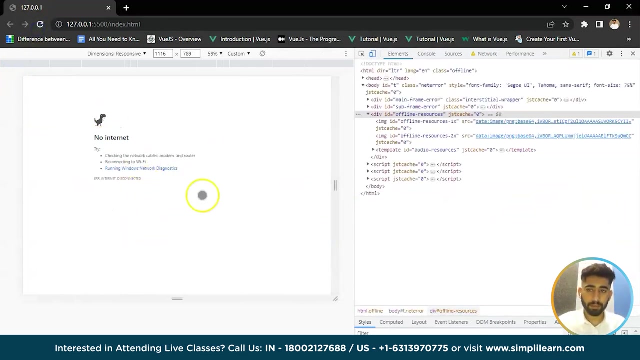 the dev. we can add that, surely? so we'll do that div dot in the day text. hello from simply them. or we can also write subscribe to simply learn. okay, and i will save it as you can see. there you will find there's no, nothing working. it's an error, not an issue. we will find that dev because you will. 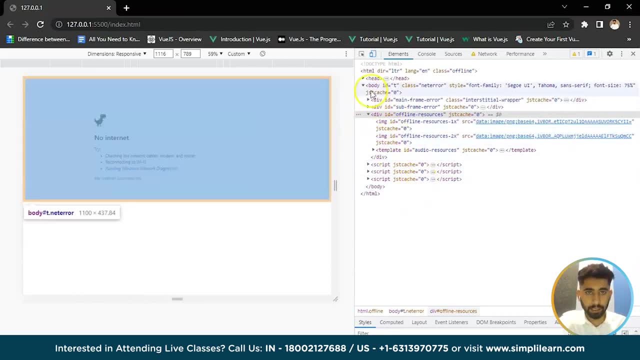 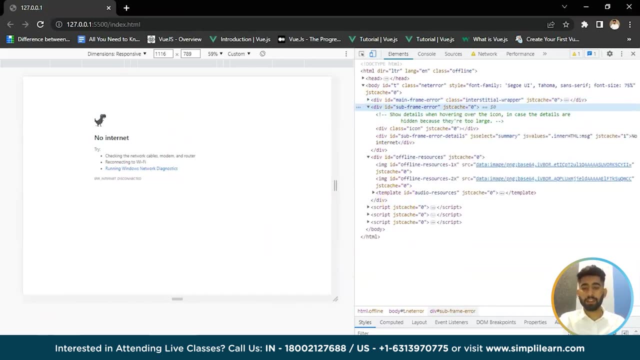 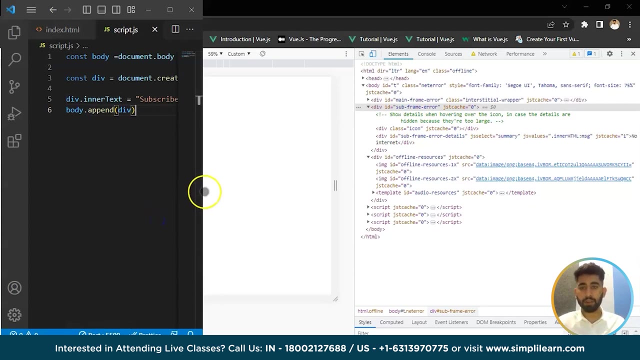 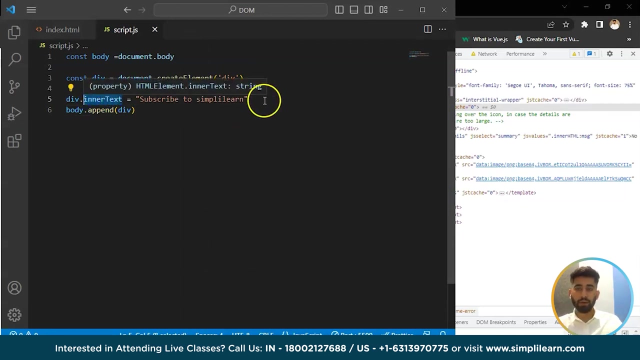 you will find that dev inside this. right, this is the mainframe. inside this there is an id, and all right. so let's now print something on the screen. right for that, i'm gonna add a change in this inner text, or we can also write another line and we can commit this. 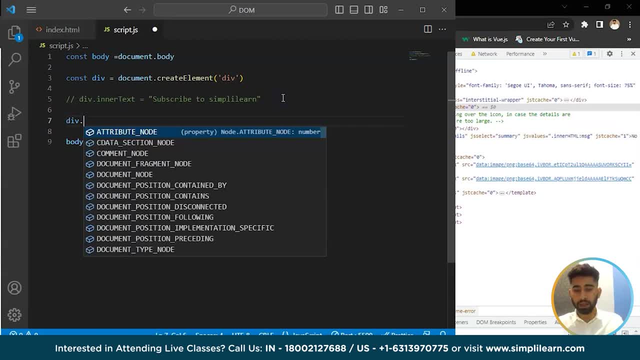 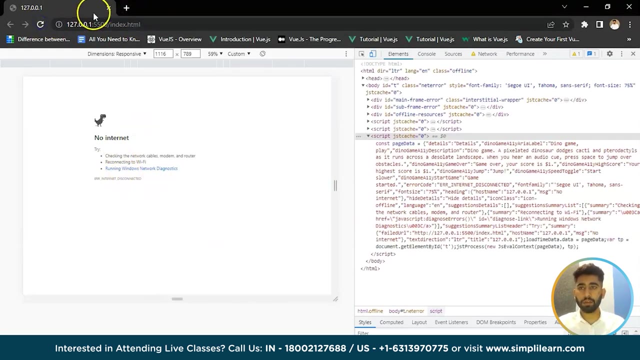 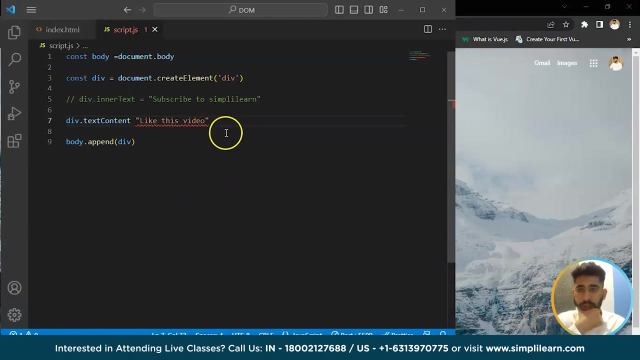 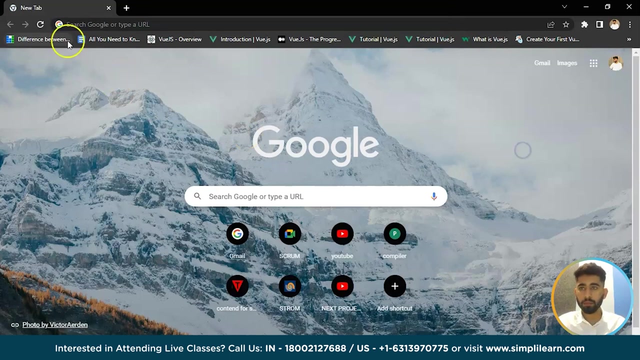 and you can write dev dot text content and i will write like this video and we'll save it and you will see this work. okay, this is not working. okay, we can start this out again. there's one error here. let me check. okay, yeah, let's just open this one, go live. 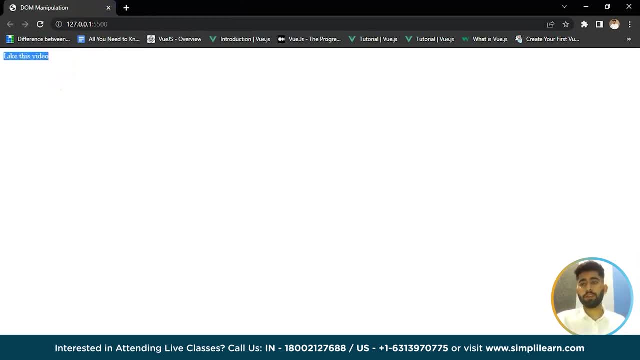 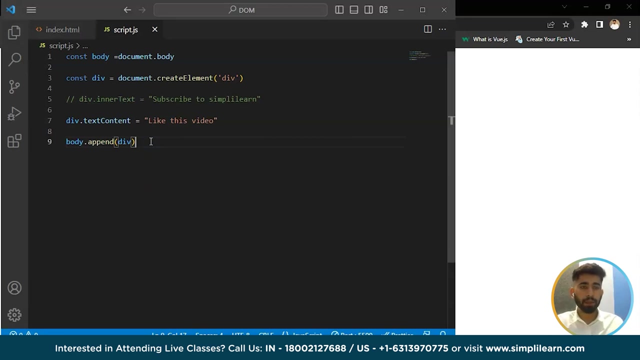 yeah, as you can see, it's showing like this video. now we will see how to modify the element so we can modify the text from. by using so many other functions also, we can add here it like using text content and all. by using this we can add and modify the text. 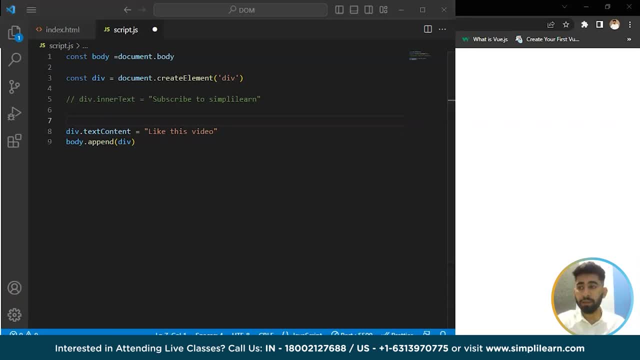 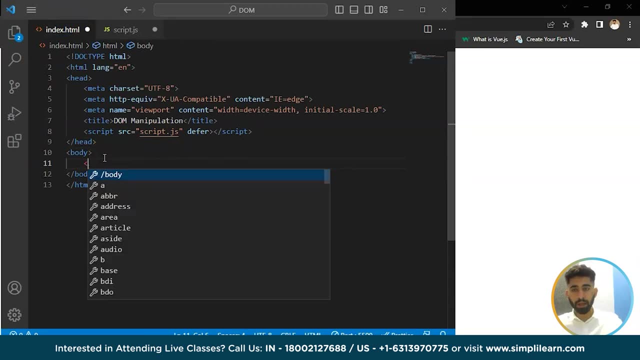 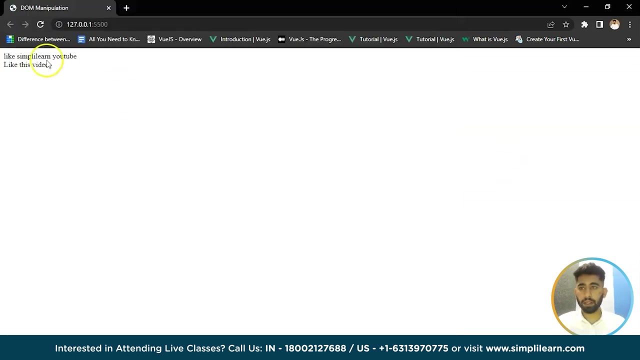 right as now we are seeing modify element text. so let's see, i'll open my html page and inside the body i'll take span like here: right, like one other youtube, right, it's just a dummy text. so, as you can see, it's showing like simply on youtube, like this video. because of that. 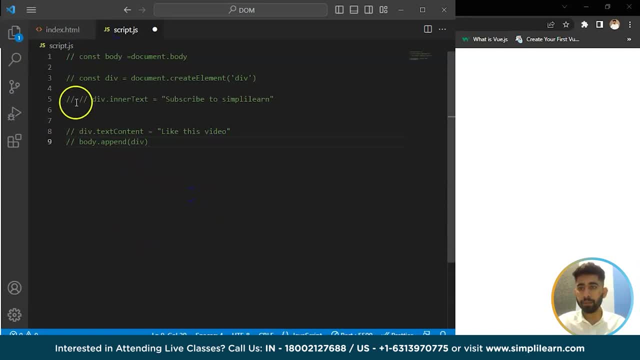 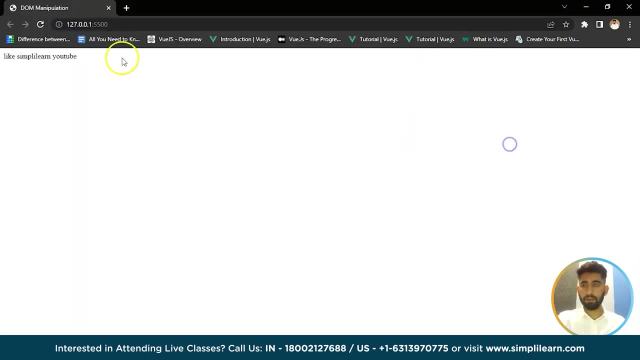 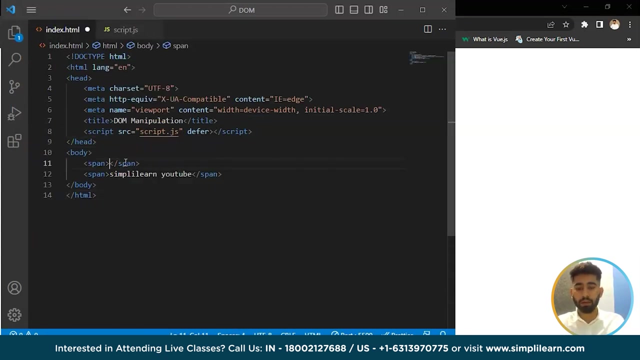 this script tag, so let's comment it down for now. okay, and let's see. it's like simply on youtube. okay, now we can write hello for making sense. okay, now, if i want to give, okay, we'll change this from give some styling to this, simply to modify element text. we are seeing it right. 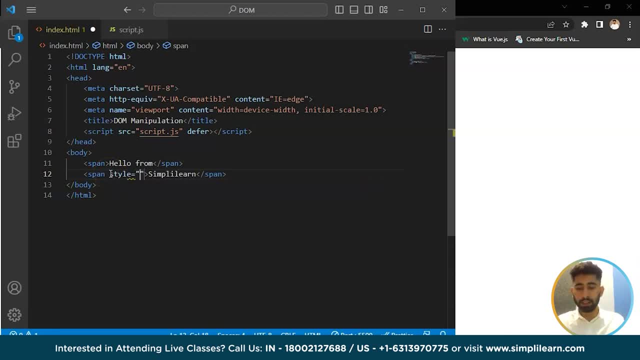 so here we'll write style and it's type the style i'm going to write. display. so here we'll write style and it's type the style i'm going to write. display. so here we'll write style and inside the display i'm going to right a display i'm going to write. 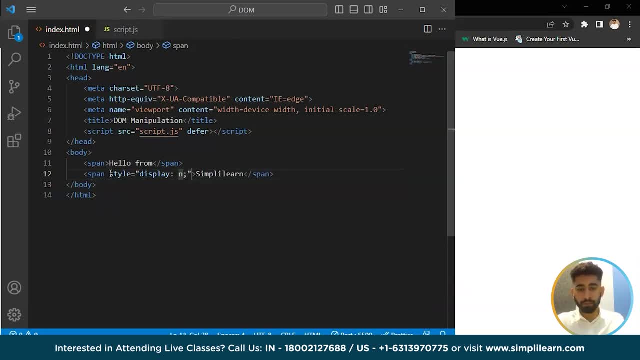 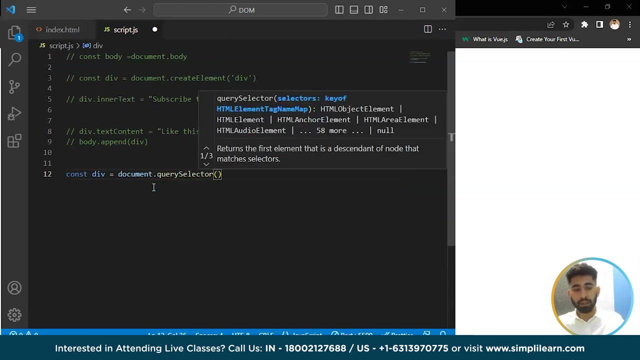 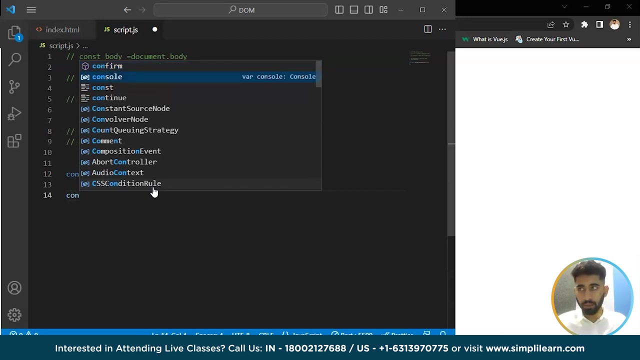 none. and now let's save this file and go to scriptjs and here we'll create one const there again and give it a document: thoughts dot- query selector. inside the query selector selector will give that a div. okay, Now here we will see two different things now, okay. 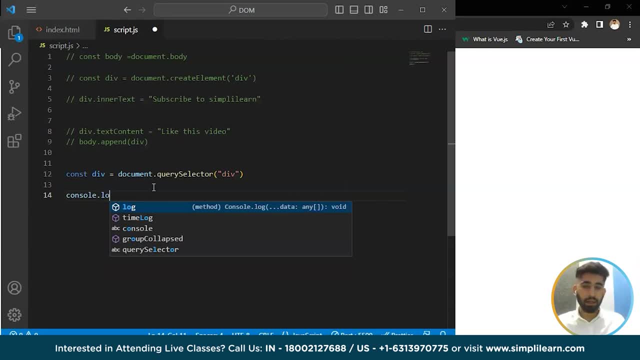 So let us see the text content and inner text. what is the difference in this modifying element text? okay, So we will write log and here we will write div dot text content. the text content is all the text that present in my body and console- dot log- and here I will give it as inner text. 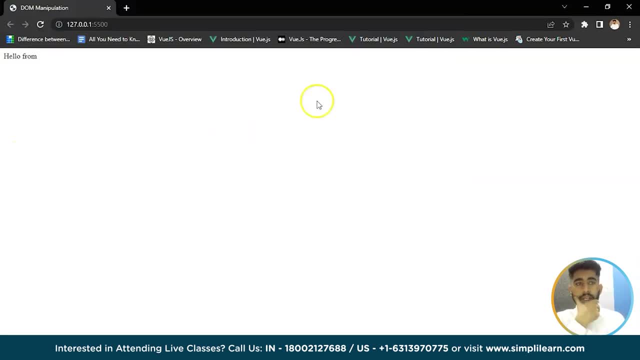 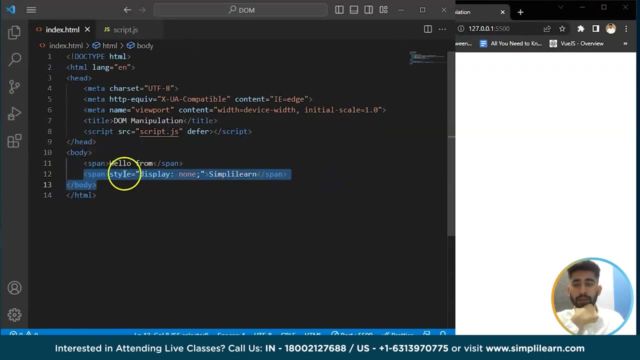 So let us save it and see what is the difference. it is showing only hello from which is this one? it is not showing me this one because I have styled it to display none. I have told it specifically to make this simply none- invisible in our screen. 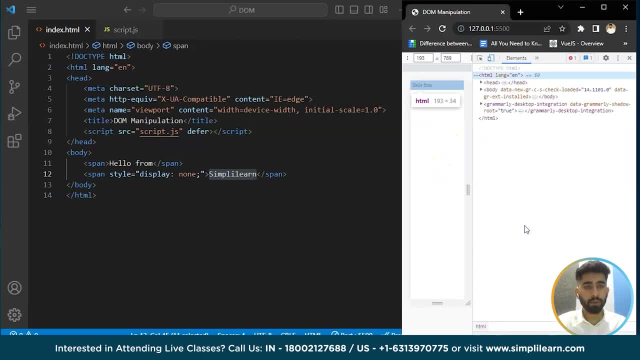 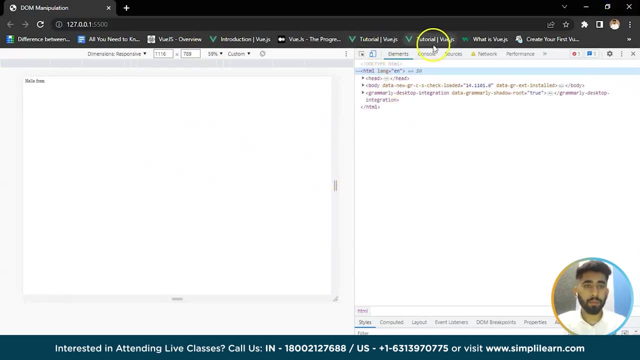 that is why it is doing this. So let us check what is the issue or what is the difference. okay, So here I will open my console and my console, you can see, cannot read properties of null. okay, So this is because, as we have written here, 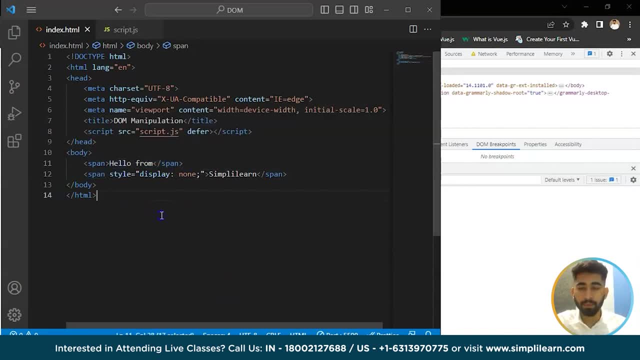 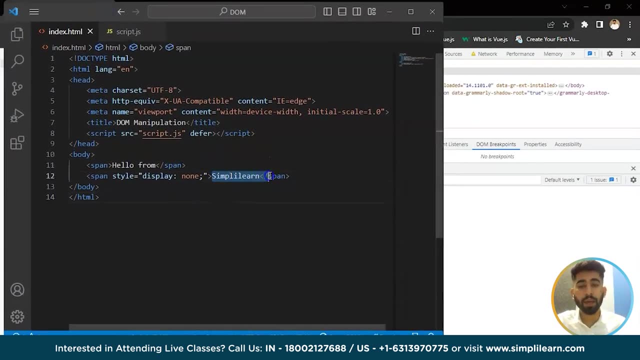 that we want spam, tell hello from. that is showing on our console page, but it is not showing this, simply none, because we have specifically given the property that we do not want this to be displayed on the screen. So in the these the difference between these two. 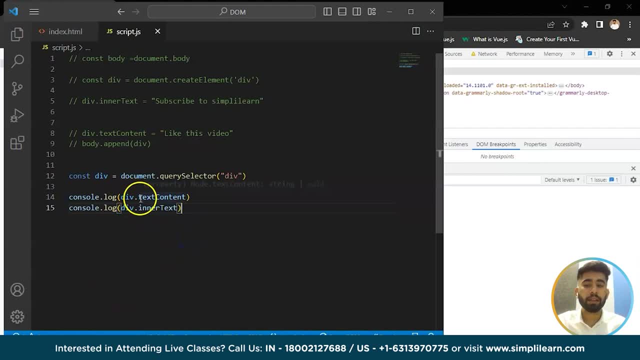 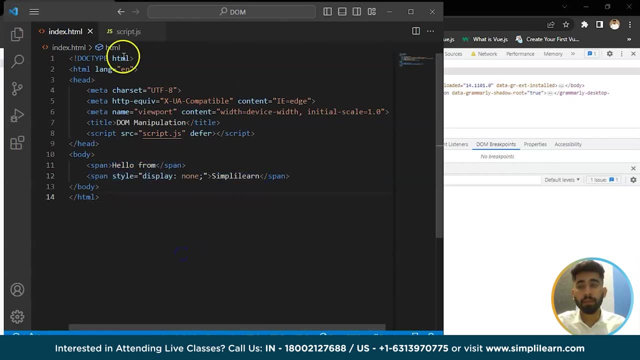 inner text and text content. the text content will print all the text that present here- hello from, simply learn. but this inner text will only print the hello from, as that you can see on the screen. so this is the main difference between the text. okay, now we will see how to modify html elements or how to add the html inside the script. 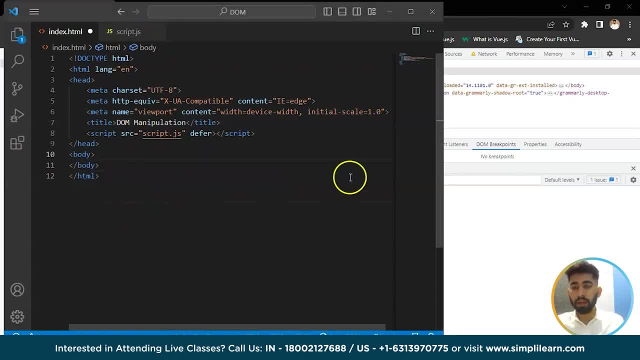 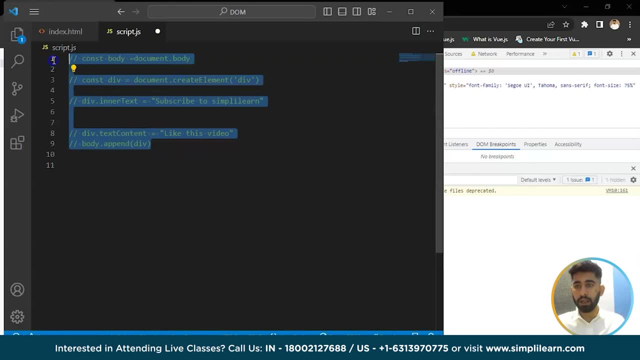 so for that, we'll remove and go back to the basic from where we started. so we'll delete this one also and we'll comment this out. okay, so, here as. let me just read one. okay, so, as here we are using in a text- we will first give it a strong to make this one. 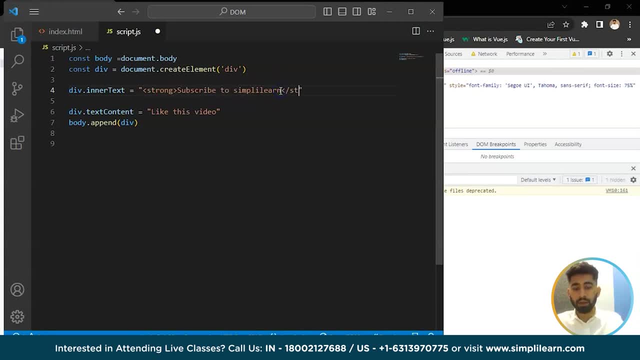 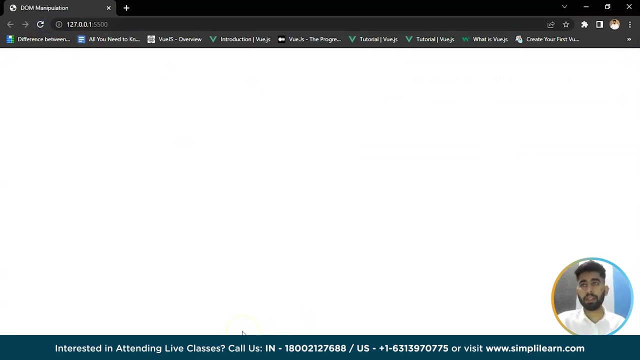 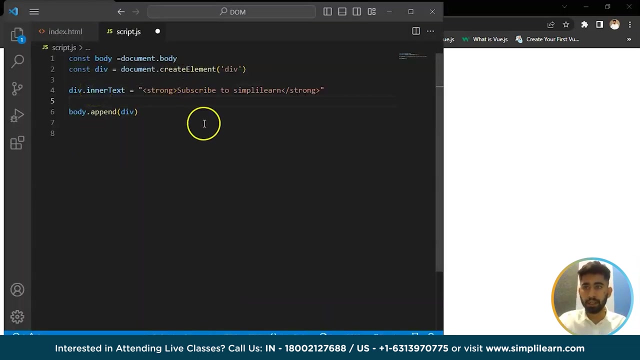 old right, and here we will close this strong tag and we'll write this: remove this from inner text. okay, let's save it and delete the console and refresh this page. as you can see, there's nothing. we'll go back here and check, okay, and we can do. append the body here, as you can see here. let me just 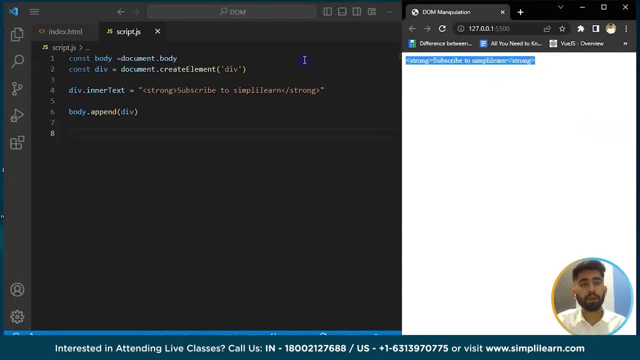 go back here. yeah, as you can see, it's just showing us all the tags of html that we don't want to see, as it is thinking it's a string. so we can modify this html element by using we we cannot. firstly, i'll tell you we cannot use the inner content or anything. we'll write here inner html and save it. 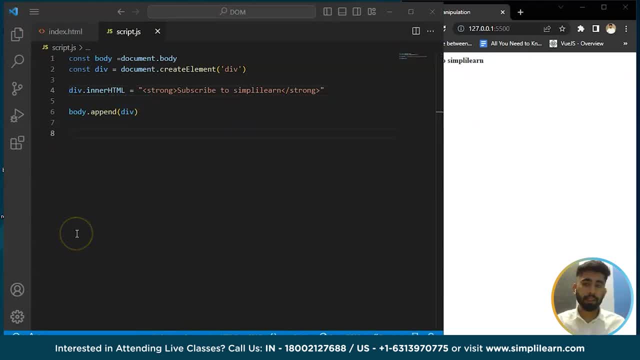 and you will see subscribe to simply learn as well. now i think you got an idea how to modify html elements so we can use, append in everything, like we can use it in the header part, body part, anywhere we can really append the elements. okay. so now let's move forward and see how to remove an. 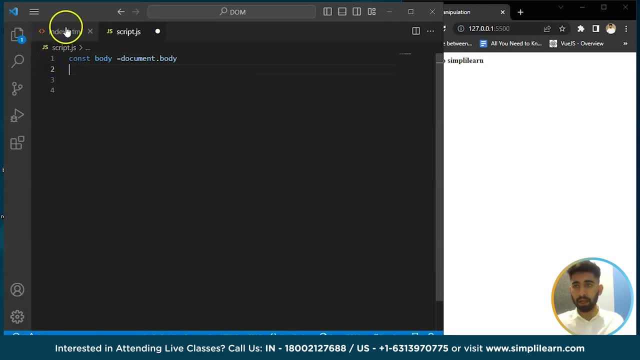 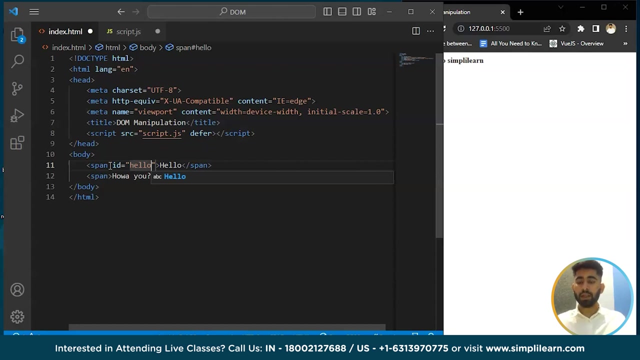 so let me just delete this part here and go to the html, and here we'll go back to that spam. and first, all right, hello, okay, and i'll take another one and here i'll write power, okay, we'll close this one and I'll give it ID. so for ID, I'll give it an ID of small IDs, so I'll give it one ABC and it's so. 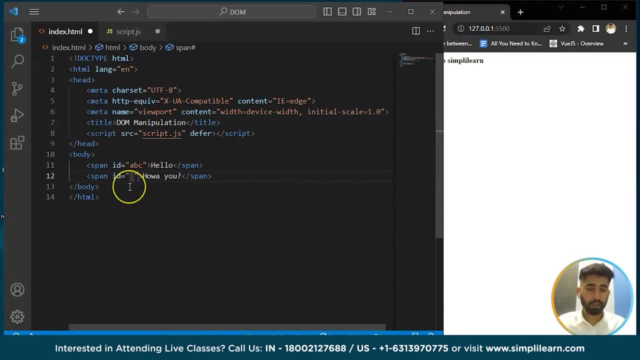 this is not recommendable to write IDs like ABC and all, because IDs is very specific. so I'll tell you about that example by giving an example. so ID is what? if we are using ID, we cannot use it after something like: I cannot change this ID after going back to some other place and if I 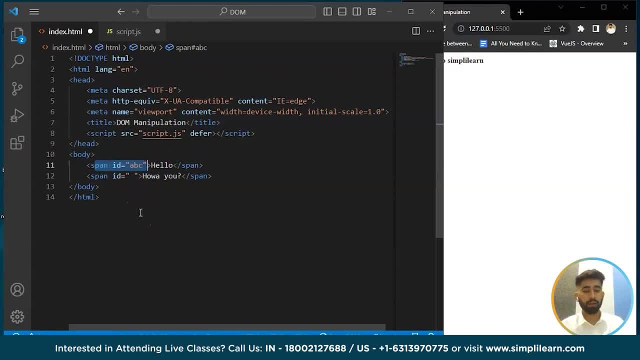 want to write this spam hello and want to change the ID of that, we cannot do that. but in classes we can do that. it's a strictly not changeable IDs. for example, in your class, if you want to, you are assigned with a specific registration number or roll number or something you cannot. 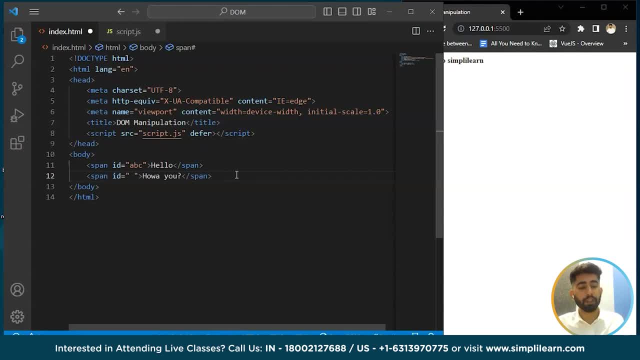 change it and nobody has the same number or the registration number as you. so this is like like an ID. you have a specific ID and in class, if you are in pursuing masters, in your class there are fifties, sixty students, or so many students say. all of the students have the same class are in. 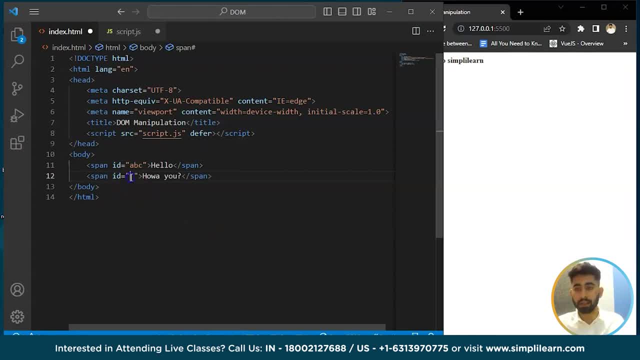 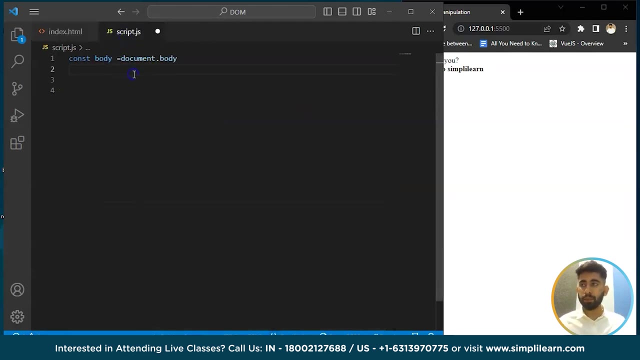 the same class rate. so data is an example of class. so here I'll write XYZ. okay, we can call. we'll call these exam. okay, see, we'll open this one and here I'll create one const def. and here I'll write document query selector- query selector. I'll write the div that we are creating here. okay, I'll just copy paste these two. 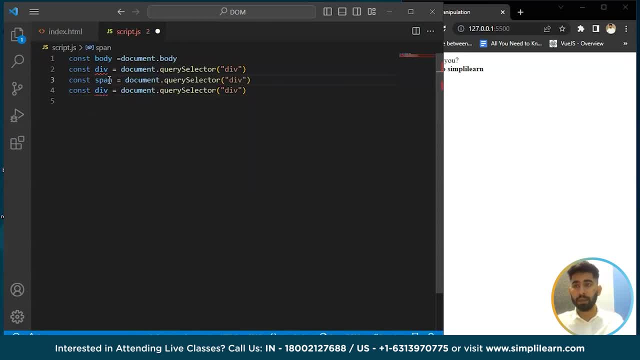 times, and here I'll write span Z and here I'll write span XYZ, XYZ, and I'll write ABC, because we have given them different. so to call the ID, we're going to use the method hash and here I'll write ABC, and we'll write here also a hash XYZ. 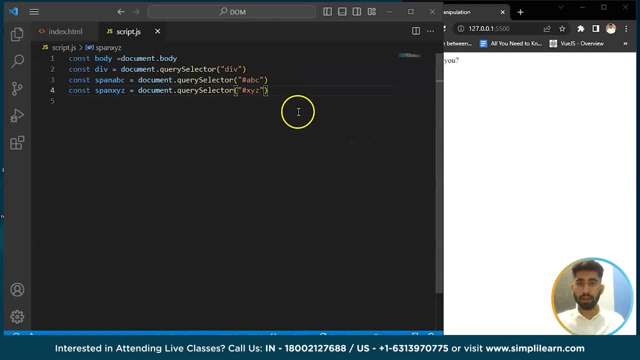 and we'll now modify the content and let's save this one and I'll see: hello, how are you? is printed on the page now. now, if you want to remove this, how are you from this? so what we can do is we can remove this element by just writing span remove and you will see. 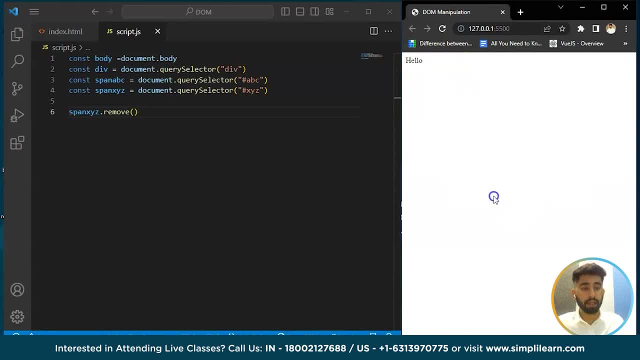 it will go out, and if you'll inspect it, you will still not find that XYZ right. this is the how. this is how you can remove the element. so we can also remove the element from the term by using remove child method. so for that we'll here write. I'll show you. 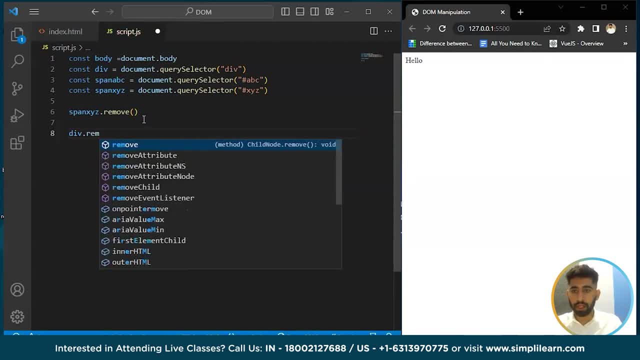 def dot: remove child. here we'll write: okay, it was XYZ, let's file comment this down. you'll see it's showing that. but let's write here: spam ABC. and it's not working. let me check this. remove child is not working, but I'll tell you about this method. so this method will only remove the child element from that. 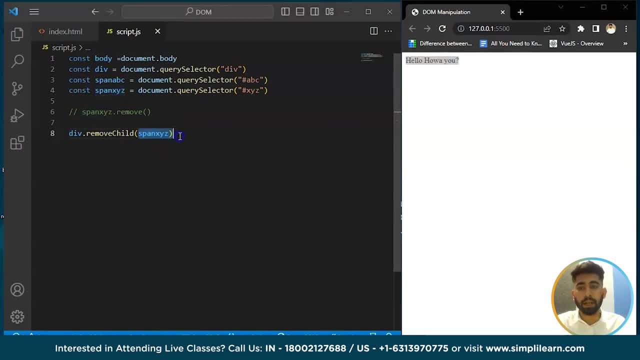 class from this. only the method that we have called will get removed. I'll always use this method only, but you can also remove. use that, this one, the remove child or append or any method that you want. you can also check out the documentation about this document: object model. it's very cool. 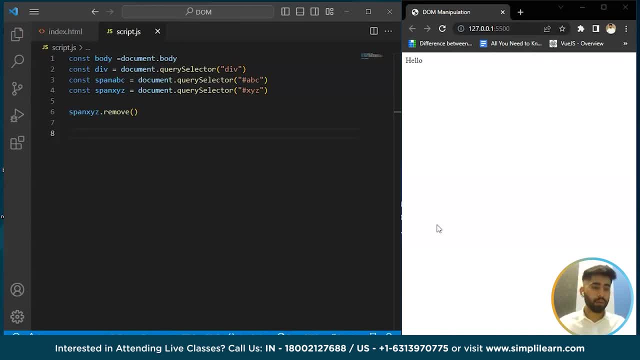 okay. so then now the last thing I want to talk about is how to modify elements in the styles. now we'll see how to directly modify any property of an element, right. so so, property wise, it's like style properties are very essential. or two way to access any CSS right.